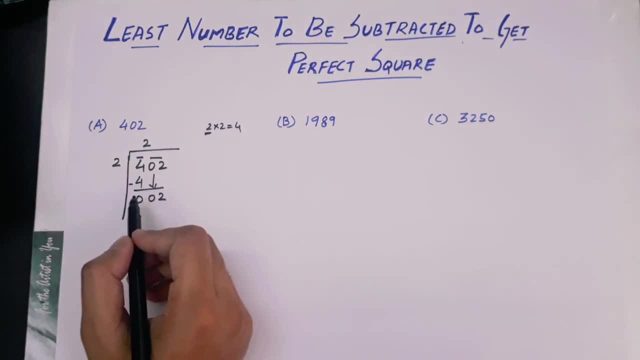 Now it is 2.. Double of 2 or twice of 2 is 2.. So it is 4.. Now, along with the 4,, I have to select one more digit, such a way that this digit in the divisor and the new digit in the quotient will be same. 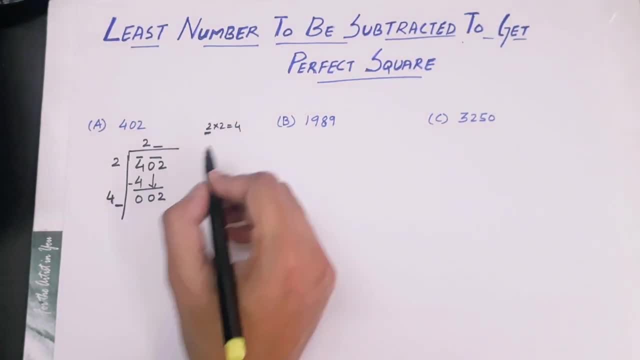 I will show you Like I can take 1. Like 41 multiplied by 1. See, I am taking both numbers, same 1 and 1. So I will get again 41. But here I have a number 2.. 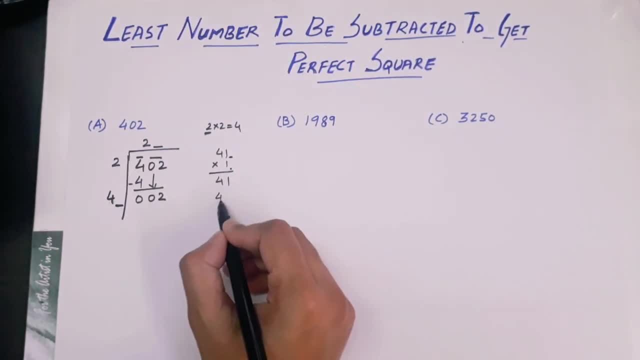 So the only option I can take is 1.. So the only option I can take is 0.. So 4 and 0 multiplied by 0, which is 40 zeros 0, we will get. So here I will take 0 and here also I will write 0. 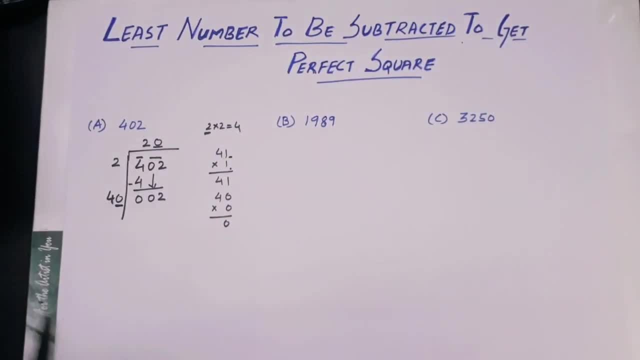 I have shown the exact how to do a division method in one of my videos. You can follow that video Here. I am just explaining in a simple way. So we will get 0 subtracted, We will get 2.. So my remainder is 2.. 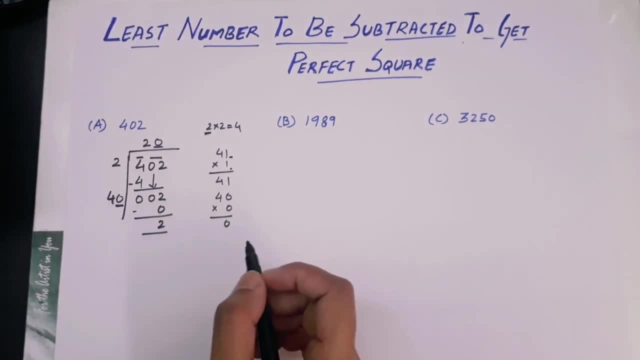 So the question they are asked is: what is the least number to be subtracted to get perfect square? So the least number is your remainder, which is 2.. So you have to subtract 2 from the 402.. So 402 minus 2.. 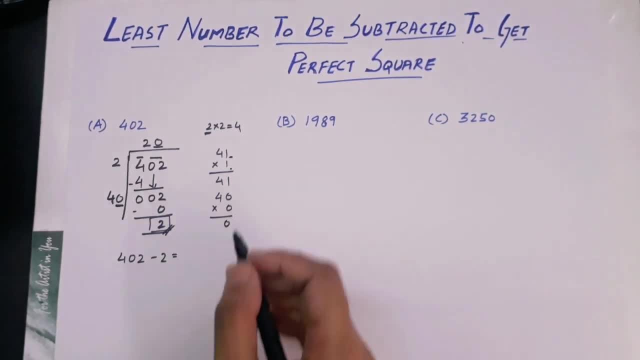 Simple concept: Do a long division or division method And then whatever remainder you are getting, that you have to subtract from the given number. I will get 400. And we know that 400 is a perfect square And square root of 400 is the same question to what we got. 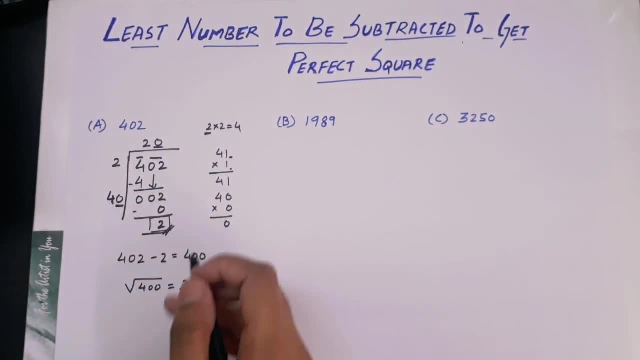 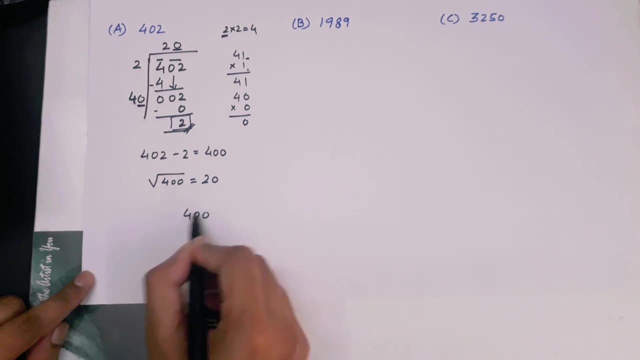 Which is 20.. We can do a long division. You can check it out. I will just show you how to cross check your answer. So I am taking a 400.. I am going to perform a long division. Pair up a number. 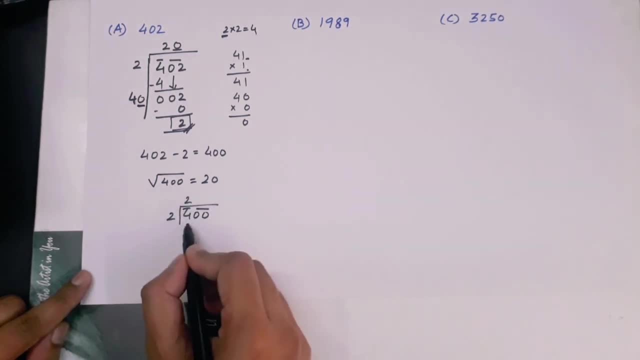 And here again, 2.. Choose a 4. Subtract it 0.. Drop the zeros. Take a twice of 2. Which is 4.. So along with 4, I should take 0.. So 40 into 0 will be 0.. 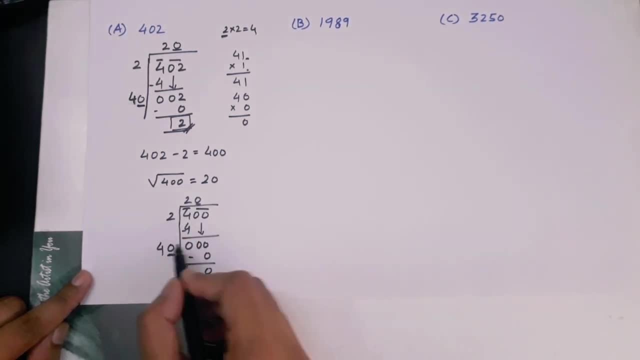 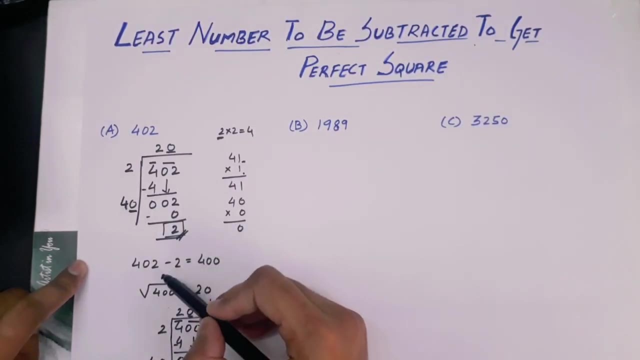 I have taken same number, 0 and 0. here I got 0. So we can say square root of 40 is 20.. So it is very simple: Do a long division method. Whatever remainder you are getting, subtract it from it. 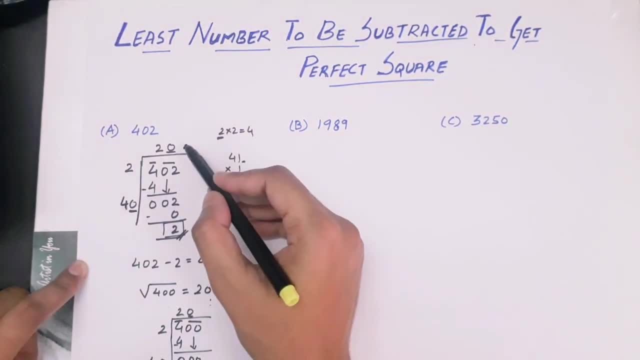 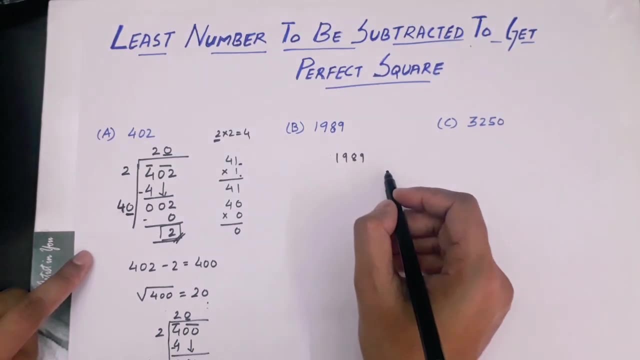 And the number you got is a perfect square, And square root of that number will be the question I will perform, For example, 1989.. First step is do a pairing from the right side. So this is my first pair. 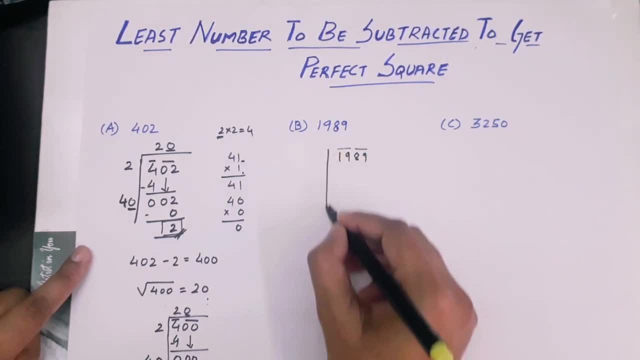 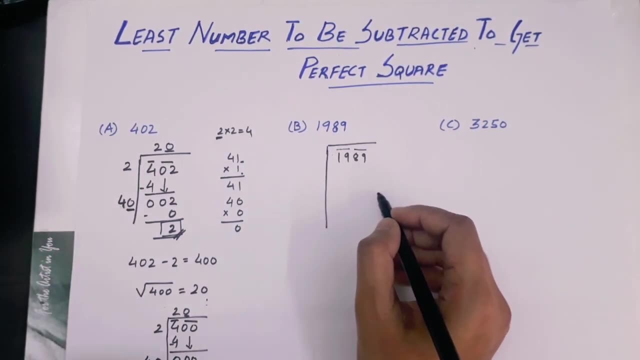 And second pair. Now let's do a long division. So the very first step is We have to check for the perfect square Nearest to 19.. So 19 is not perfect square Nearest to it is 16.. 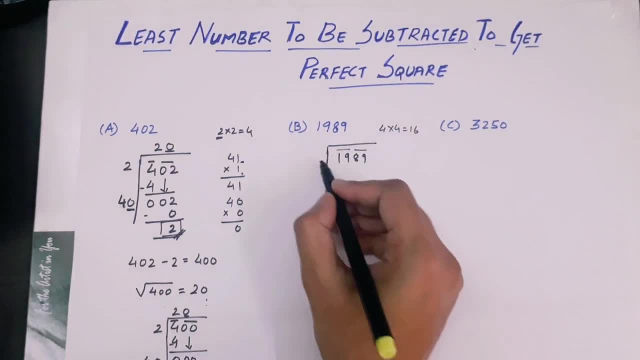 4 x 4 is 16.. So I will take 4.. 4 is 16.. Then my remainder will be 3.. Drop this 89. You have to drop both the numbers 89. Because they are in pair. 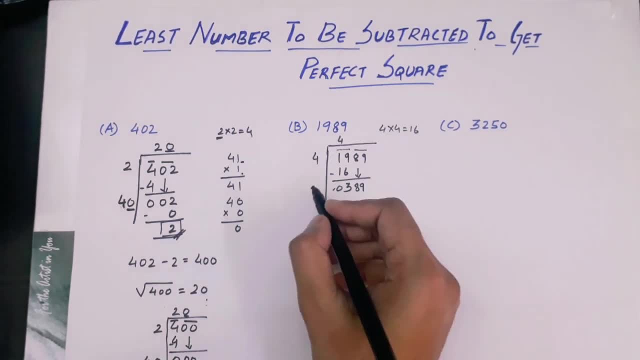 Now, second step: Choose a divisor Such a way that first digit will be twice of 4., Which is 8. Along with 8.. I have to select a digit: This digit and the digit in the question. The new digit in the question. 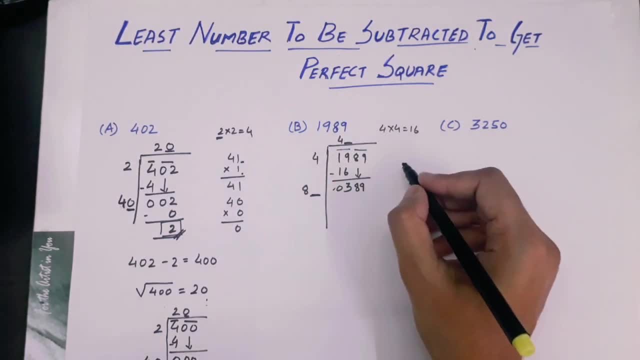 The both should be same. So I will try few methods Few numbers to just check it out Whether I am getting a number near to 389 or not. So let me take 82.. 2. So I will get 4.. 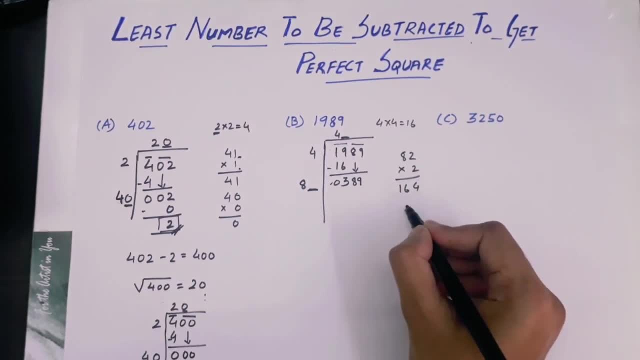 164.. It is quite small So I will just increase the number. I will take 84.. See, I am taking both numbers same here, So I will get 336.. Quite near to 389.. But I will check for 5.. 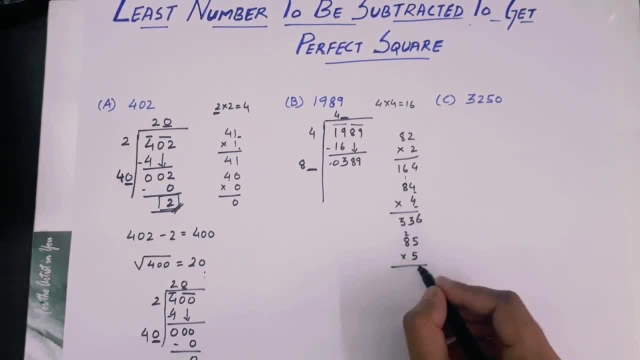 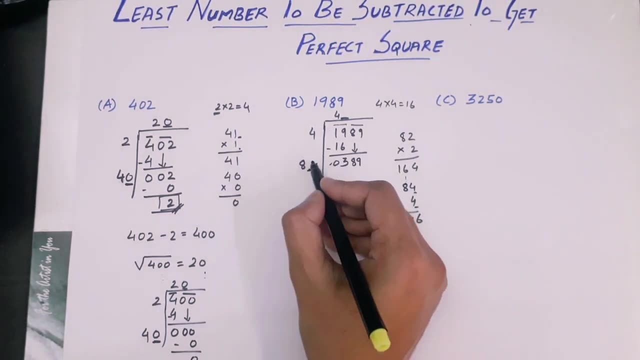 So 85.. 25.. 42.. So 425 is quite larger than 389.. So I will go for 4.. So 84.. 4. Is giving me 336.. Now, subtracted, 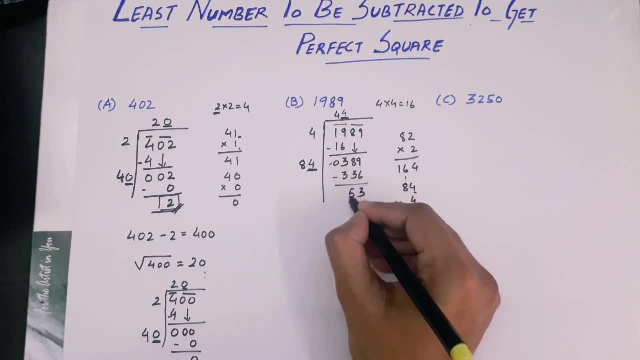 We will get 3.. And then 53 we are getting. So I have to subtract 53.. It is my remainder, So 1989.. Subtracted 53. Which will be 936.. 1936.. 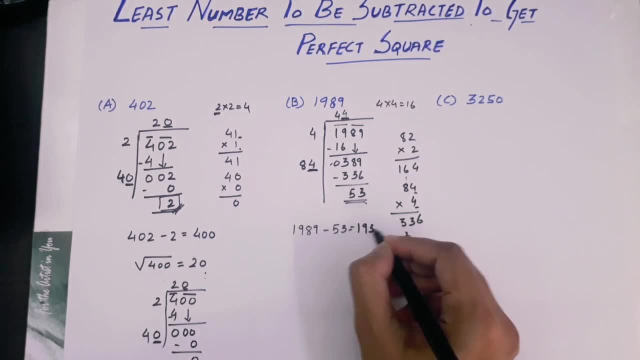 So square root of 1936. Will be: Whatever question we got Write down, That's it. You can cross check by dividing, By doing a long division method, Whether the answer will be correct, Whatever question we are getting. 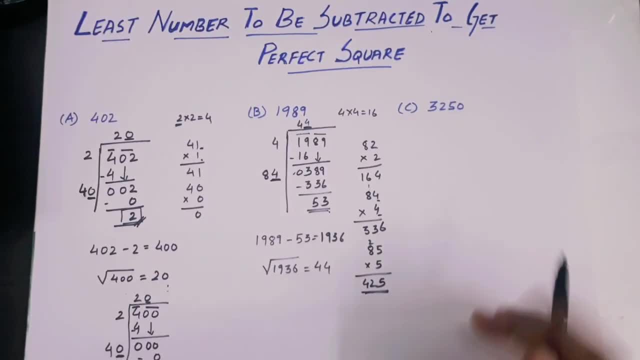 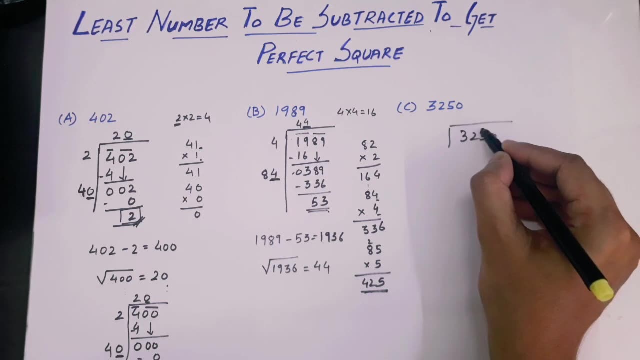 That will be the answer. So we will do the last problem. So here we go. So first 3, 2,, 5, 0.. I am going to first pair up. 50 is one pair. 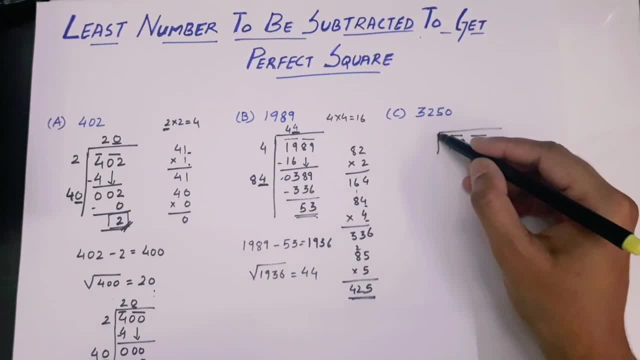 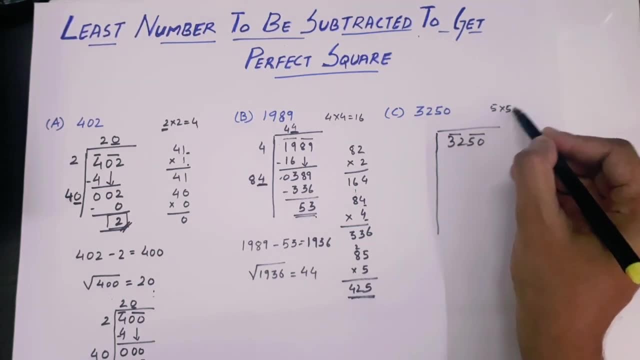 32 is one pair, Then I have to find out a perfect square Near to 32 or equal to 32.. Since 32 is not perfect square, So nearest to it will be 5,. 5 is 25.. 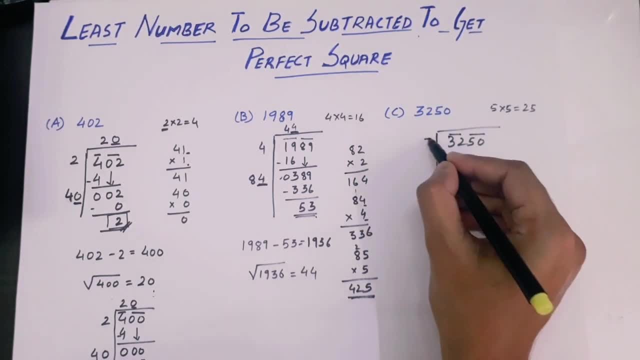 Because 6x is 36.. It is larger, 5 is a 25. Subtract it, We will get 7., And then Drop 50.. So we have 750.. As a new dividend, Now take us: 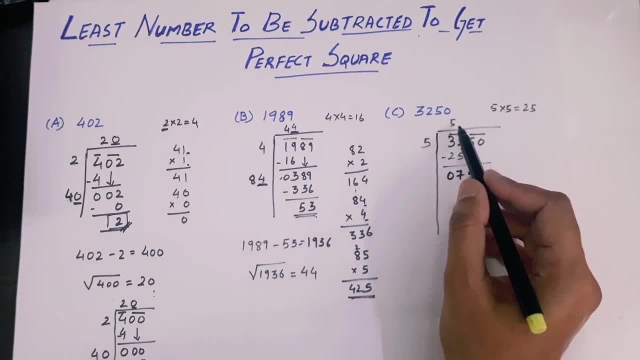 For the new divisor, Take a twice of the current question, Which is 5.. So double or twice of 5 will be 10.. So along with 10. I have to find a new digit, So let's try a different number. 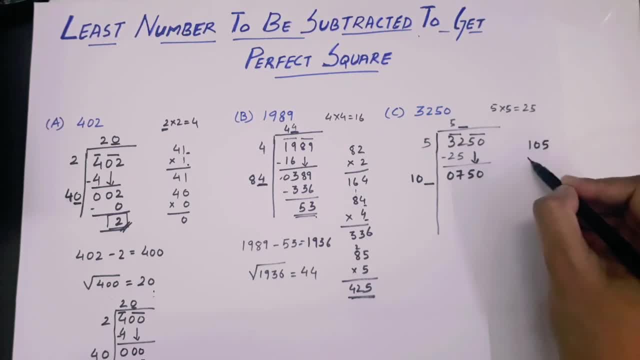 So I will take 105 x 5.. I am just doing a trial and error method. We have to just bring the number Near to 750 or equal to 750. But we will not get equal Because they are not perfect square. 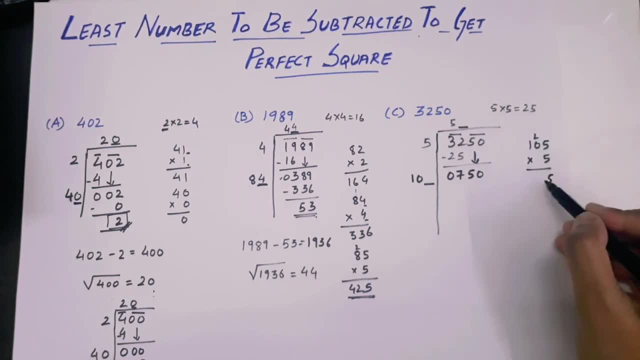 So we have to find out less than that. So 5 x 5 is 25.. Then 2.. 5 x 25 is quite far. I will try for the next number, Let me take 7.. So 7 x 7 is 49.. 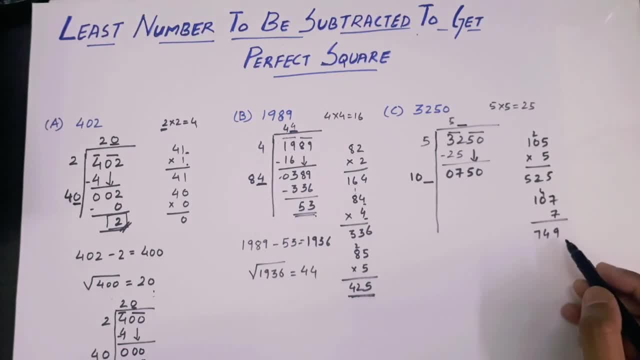 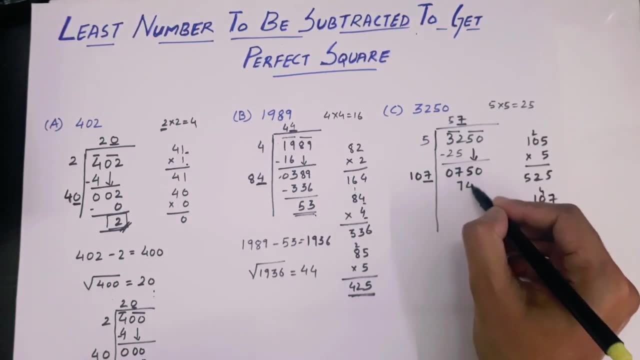 Then 4.. Then 7.. It is near to 750.. So we will take 707.. And multiplied by 7., We are getting 749.. So your remainder will be 1.. So we need to subtract 1.. 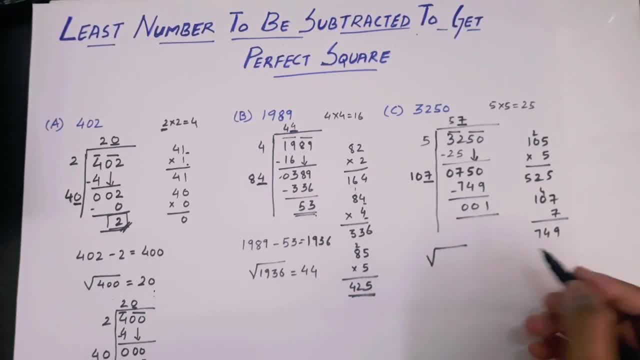 From this. So square root of. I forgot to subtract, So 3,, 2,, 5,, 0.. Subtract 1. We will get 3,, 2,, 4,, 9.. And square root of. 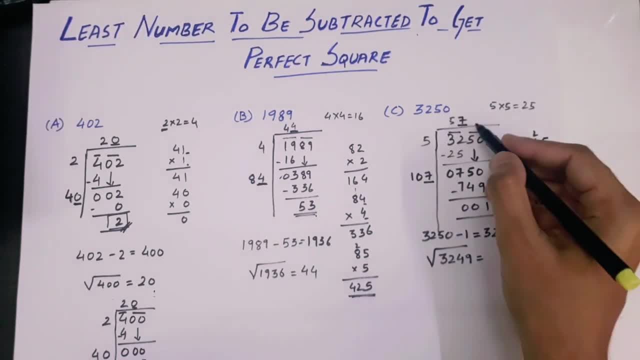 3,, 2,, 4, 9.. Will be your quotient, Which is 57.. That's it. So this is how we have to do it. If they ask you What is the smallest number to be subtracted, 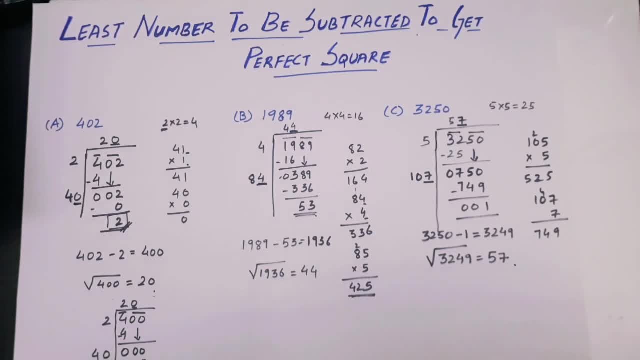 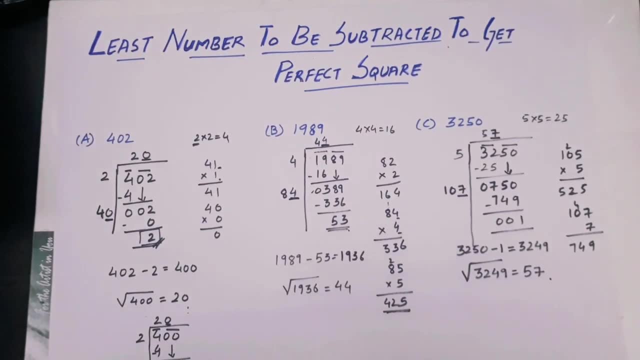 Go for division method And whatever remainder we are getting, We have to subtract that from the given number And you will get the perfect square. So this is how we can do it. Thank you so much for watching. 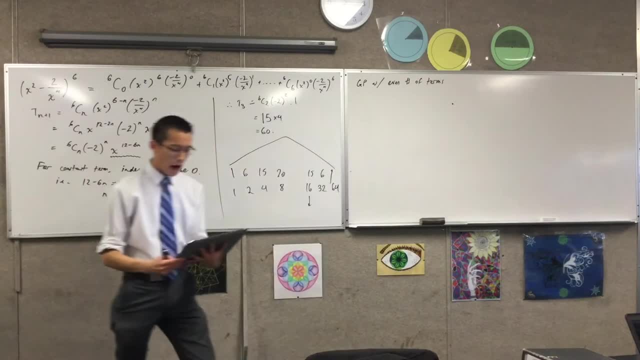 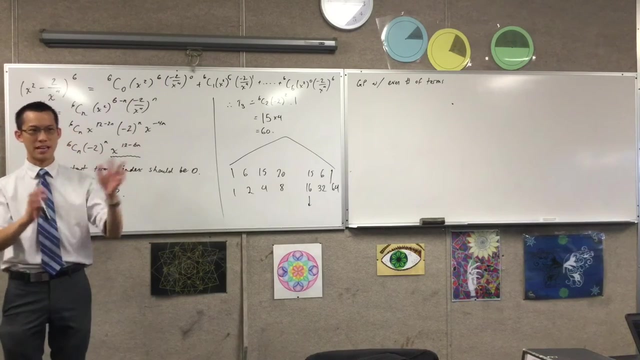 Question says this is the exact wording. actually a geometric series has an even number of terms. The sum of the whole series is 5 times the sum of the terms in the odd places. Let me say that again: GP- even number of terms.